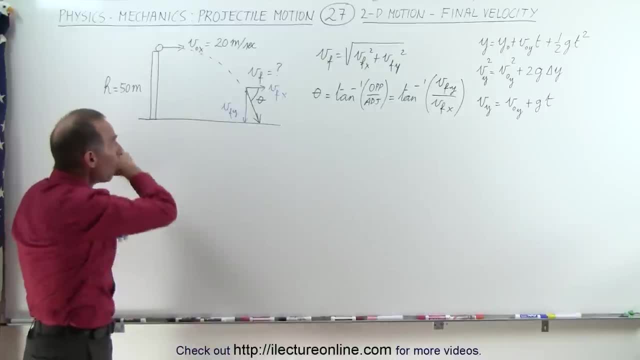 changes because there are no forces acting on that object while it's flying to the air in the x direction. The y direction- yes, that's due to gravity. that will change its velocity in the y direction, but there will be no change in the velocity in the x direction because there's no 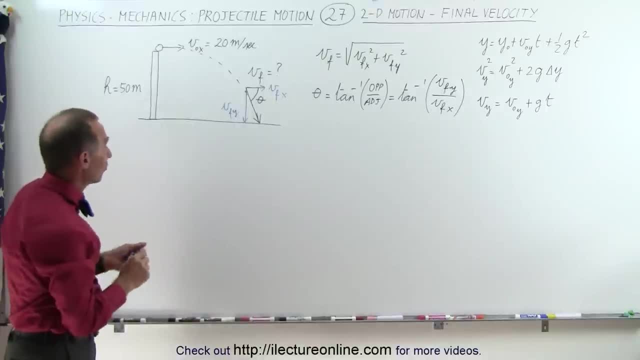 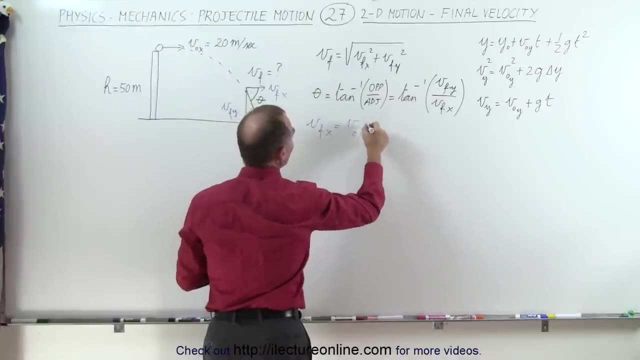 forces involved, and we're also ignoring any wind resistance. Therefore, we can say that the velocity final in the x direction equals the velocity initial in the x direction, which in this case is equal to 20 meters per second. So that makes it equal to the velocity initial in the x direction. 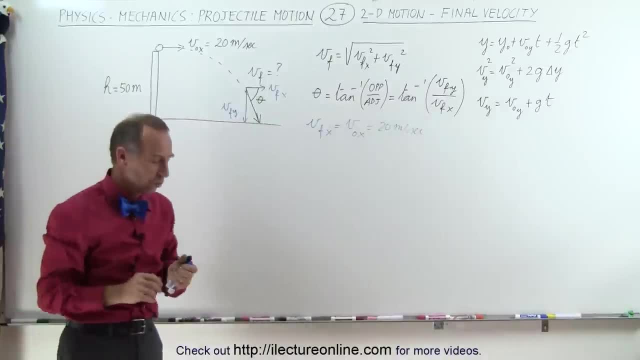 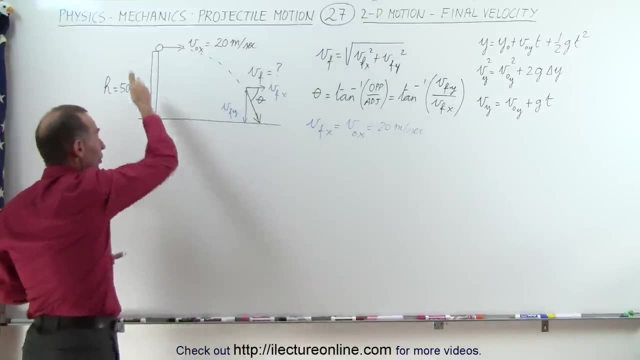 So that makes it easy. Now for the velocity in the y direction. We can do that in two ways. We can first assume that we're going to find the time in the air which depends on the vertical component, and then use that time to find the velocity in the y direction. So let's do that. 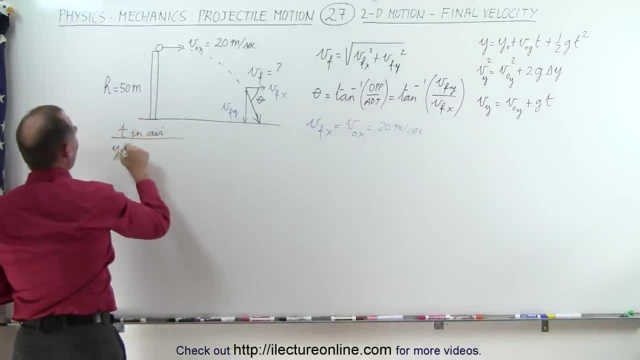 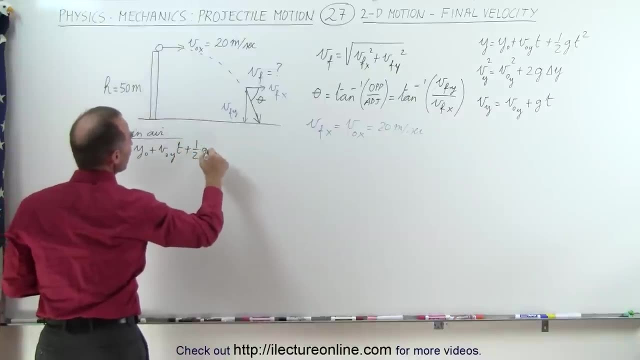 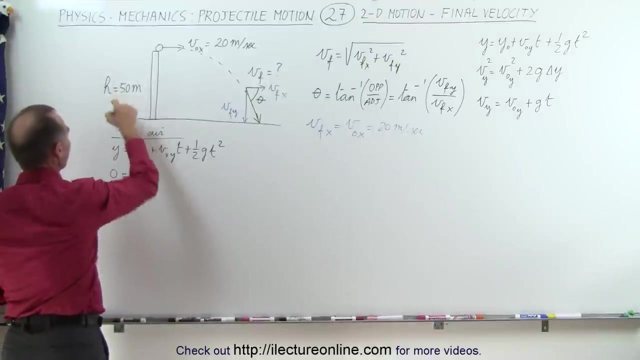 Time in the air. We use the equation: y equals y sub naught plus v sub naught in the y direction. times time plus one half. that would be g? t squared, Plugging in the numbers: Final height: zero. Initial height: 50 meters. Initial velocity in. 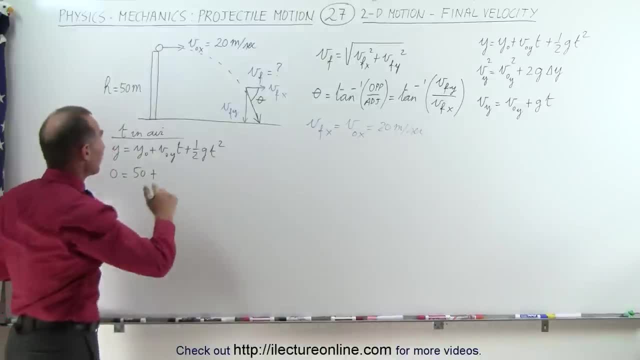 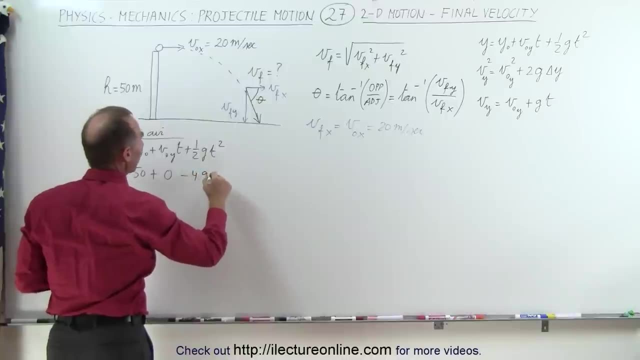 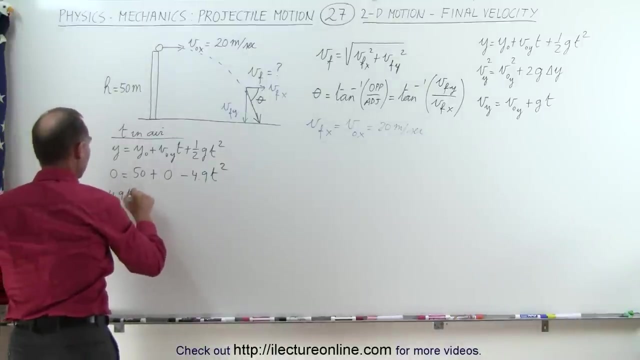 the y direction. Well, if it's thrown horizontally out, there'll be zero velocity in the y direction and then minus a half a g, which is a minus 4.9 t squared. Solving that for t, we get 4.9 t squared is equal to 50 or t is equal to the square root. 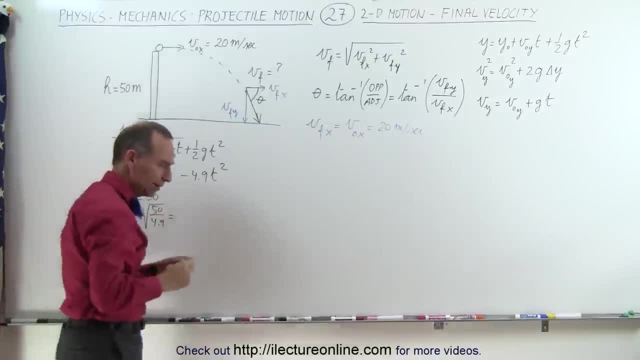 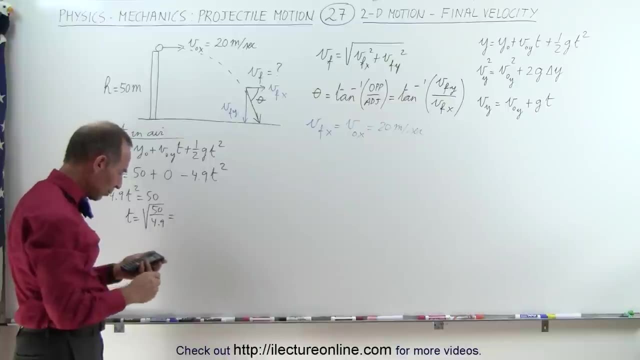 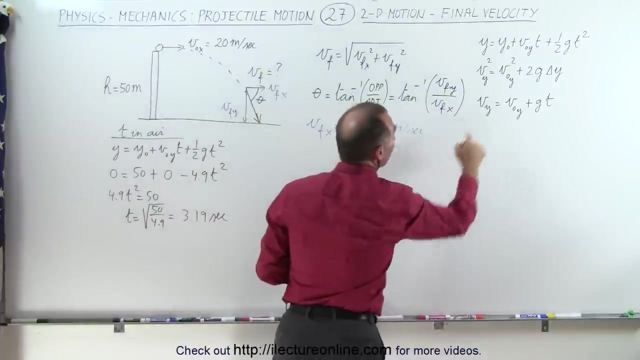 of 50 divided by 4.9.. With a calculator, let's find out what that is: equal to 50 divided by 4.9.. Take the square root and we get 3.19 seconds. If we now use the third equation over here, we can use v sub y, v in the y direction, The final v. 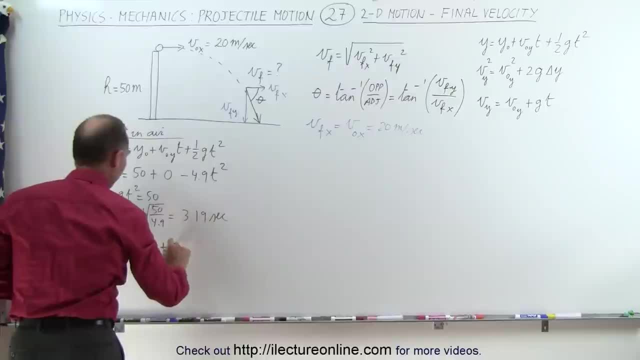 sub y is equal to v initial in the y direction, plus g times t. now that we know the time, Remember that v is equal to 0 minus 9.8 meters per second. This is equal to 0 minus 9.8 times 3.19, and so v- y. 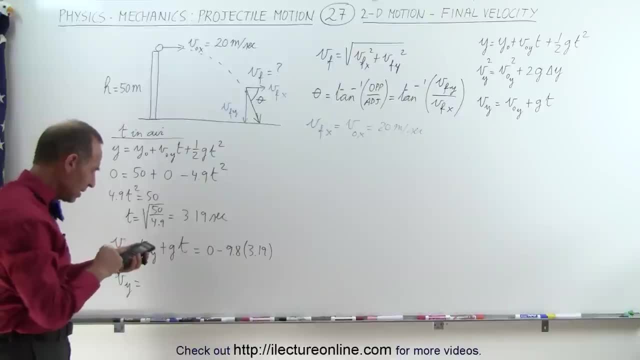 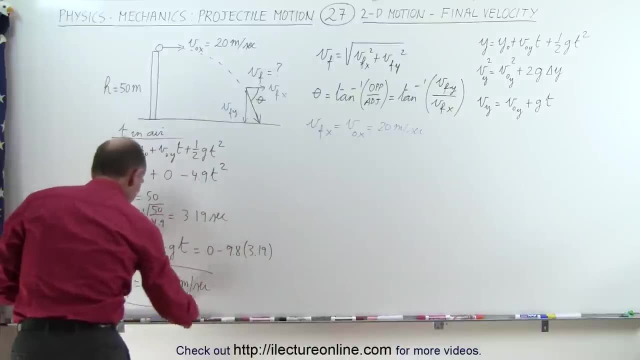 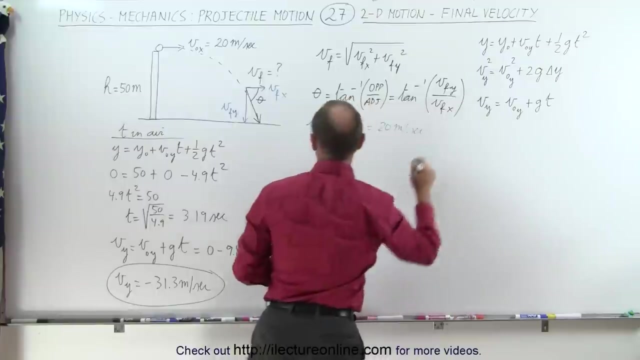 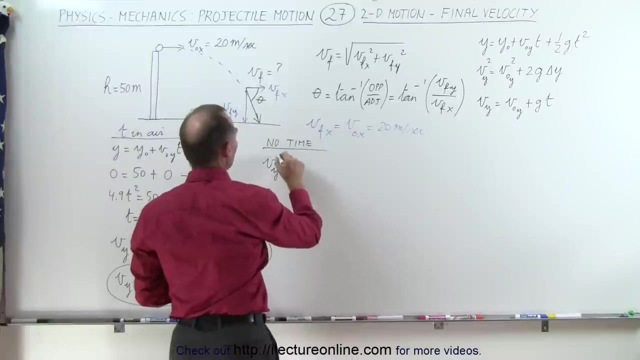 is equal to times 9.8 equals minus 31.3 meters per second. You can also solve this without finding the time in the air. We can use our second equation here. We can say that v squared, so no time. We can say that v? y squared equals v y initial squared, The initial velocity squared. 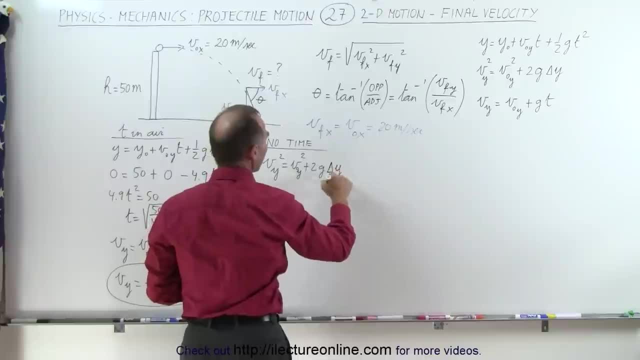 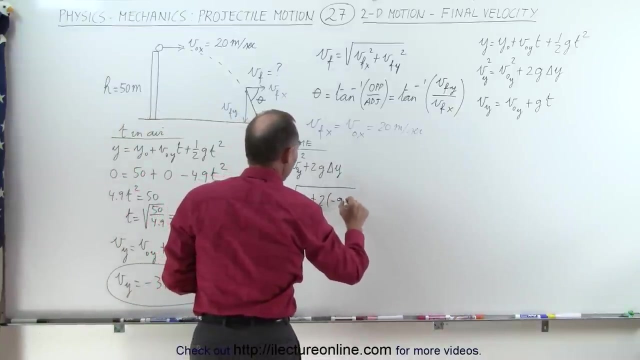 plus 2 g times delta y, That's the change in height To find a velocity, then v y is going to be equal to the square root of the initial velocity in the y direction. squared Again, the initial velocity is zero plus two times a, minus 9.8 times a minus 50.. 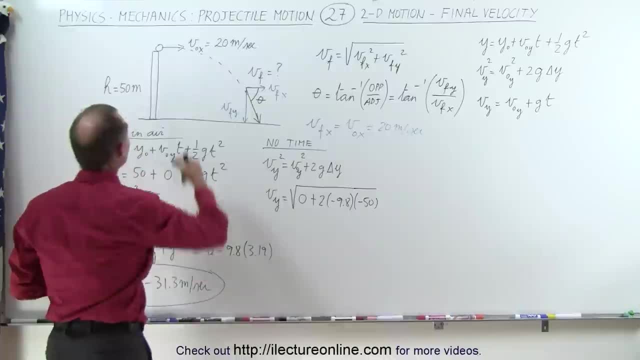 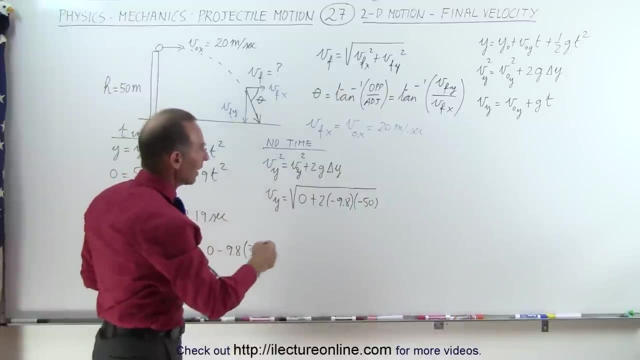 Now you say: well, why a minus 50?? Well, because the change is from 50 to zero, So that's a negative change in the height. therefore, a minus 50.. That gives us 100 times 9.8 is 980.. So the square root 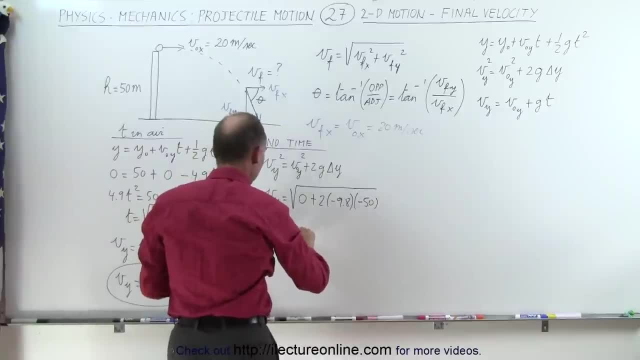 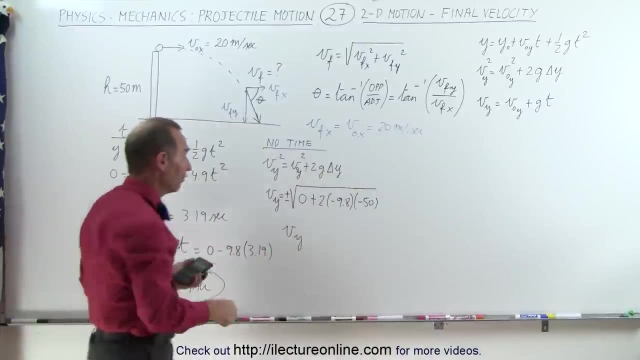 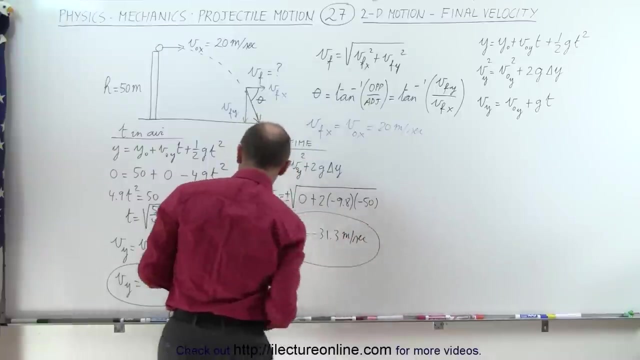 of 980 is indeed the same v sub y, And of course I should put down plus or minus, because in this case what makes sense, since it's coming down v sub y, is going to be a minus 31.3 meters per second. You can see that you can find it both ways: finding time in the air or simply using that equation. 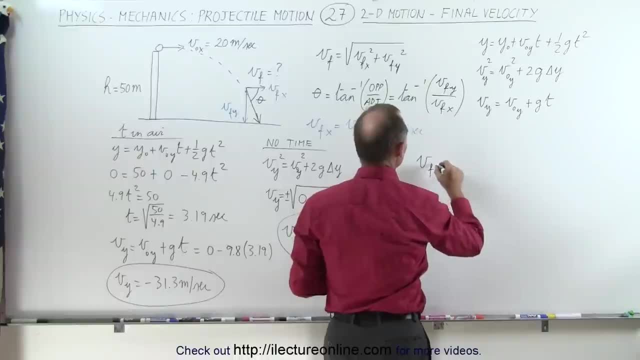 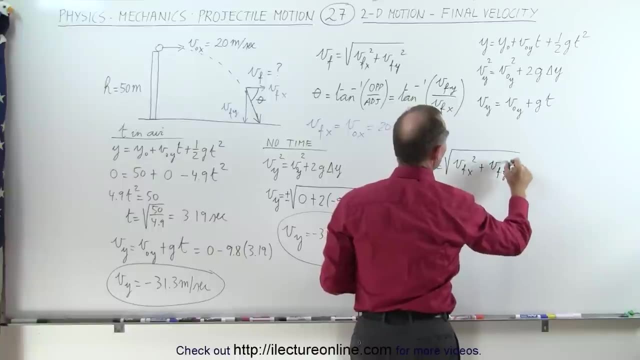 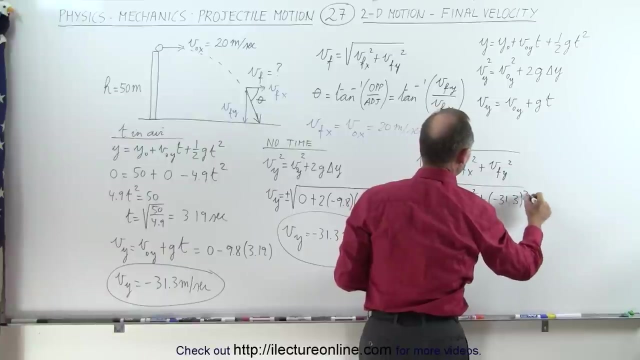 Finally, we're going to find v final. v final is equal to the square root of v final in the x direction squared, plus v final in the y direction squared. This is equal to the square root of 20 squared, plus a minus 31.3 squared. Now, here we're going to end up with a positive quantity. Why? 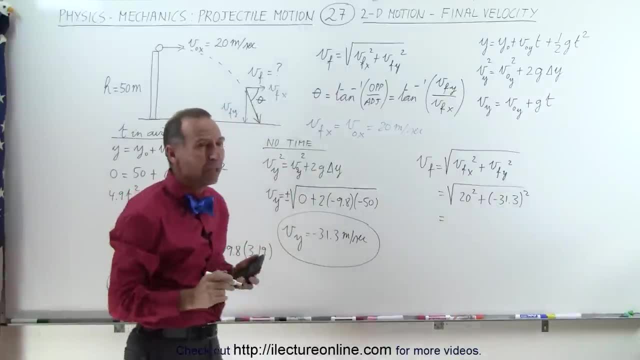 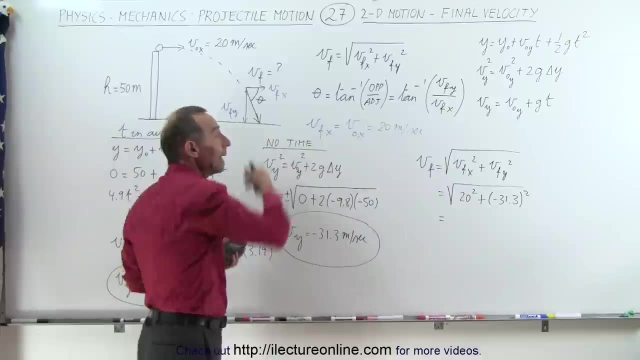 Because we're simplifying the magnitude of that final velocity. We can't really say that it's going in a negative direction because it's not going straight down, It's not going to the left, It's going at an angle. So with vectors, we're going to express it in terms of the magnitude. 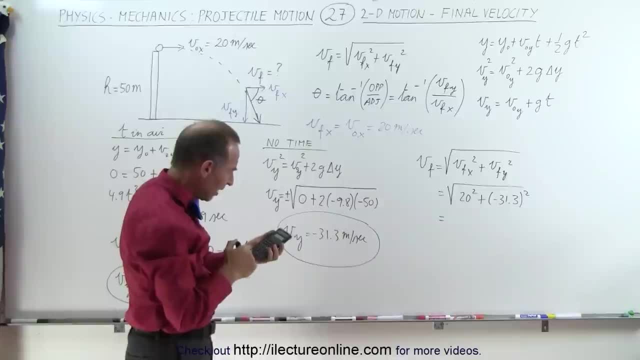 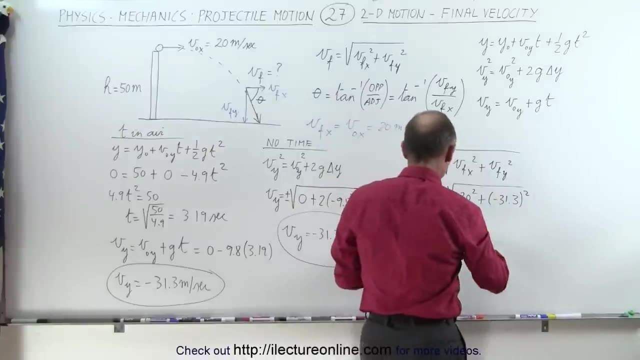 and the direction. Direction in terms of the angle. So in this case we'll take the squared plus 400.. Take the square root, we end up with 37.1 meters per second. Notice: it's going to be positive quantity because it's the magnitude of the final.